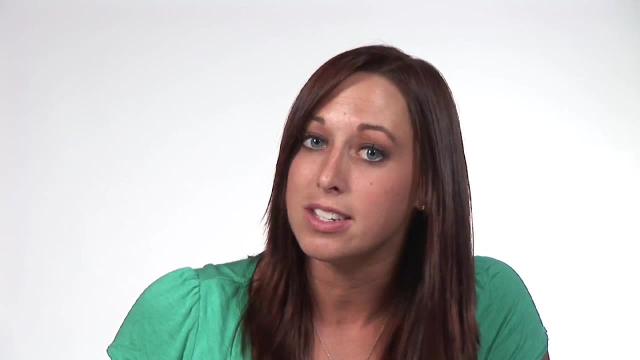 or what portion of that food or food component is providing towards your calories or daily nutrient needs. Now, a recommended daily allowance or daily nutrient allowance is the daily percentage of food that you eat Now a recommended daily allowance or daily nutrient allowance. is the daily percentage of food that you eat Now. a recommended daily allowance or daily nutrient allowance is the daily percentage of food that you eat In our Mohan Ayyar program. the recommended daily allowance or daily nutrient allowance. 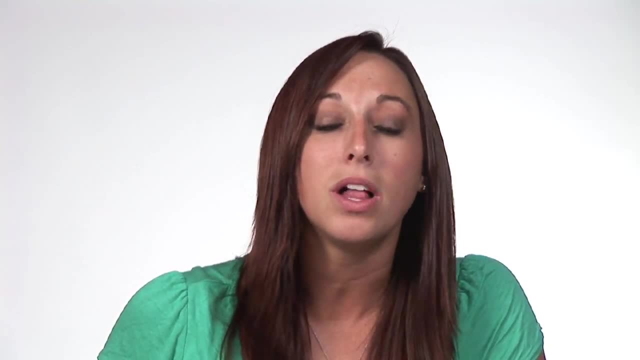 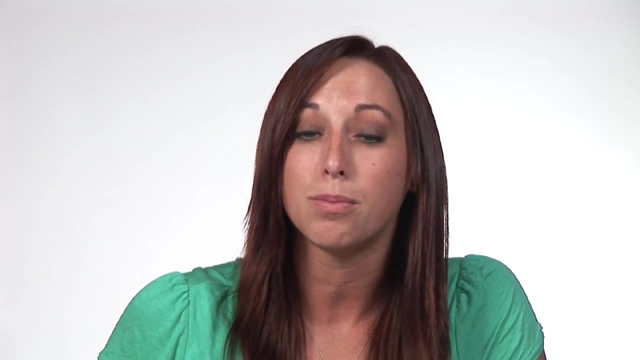 is an average of the amount of protein, carbohydrates and fat we should have, as well as the amount of vitamins and minerals we should have on a daily intake level. Now, in general, our macronutrients, or the things that provide us calories, which are the carbohydrates. 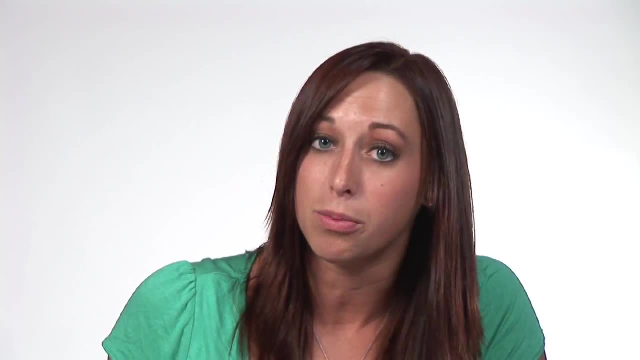 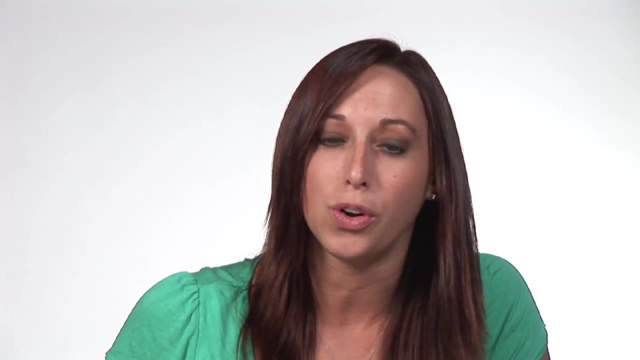 which typically you want to aim for. 50 to 60% of your diet coming from carbohydrates are fats, which really only need about 20% or so, and our protein again 20 to 30%. All with a little bit of slip and slide video between these few phrases, so we're not having 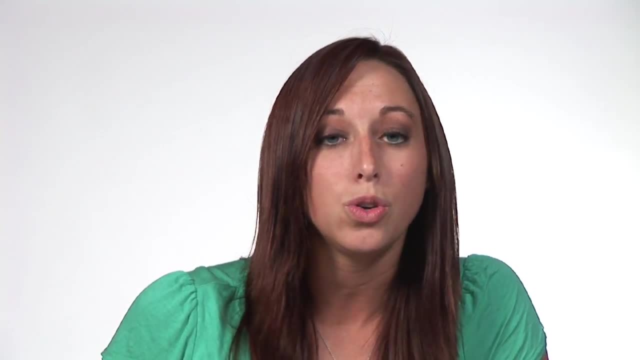 much of an artillery pound here, but the case in our health science program uses citric powder, which is the facts of molds that shape up your body. ausge exercizi liver lipido between. Now, when you look at a nutrition facts label, here I have an example We can 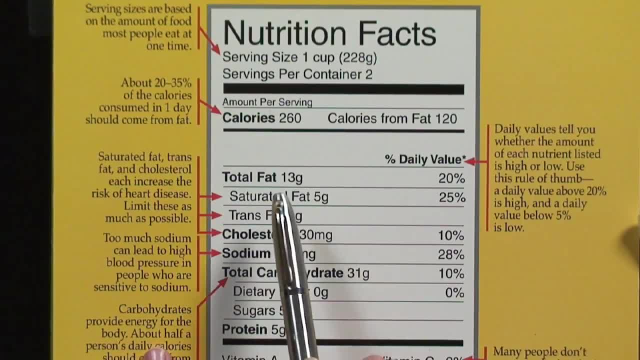 look at our total calories, which I said are combined of a few things: your fat, your carbohydrates and your protein. Now, by doing a simple percentage, you can see what percentage of those calories are coming from these different nutrients. So, for instance, they've actually calculated. 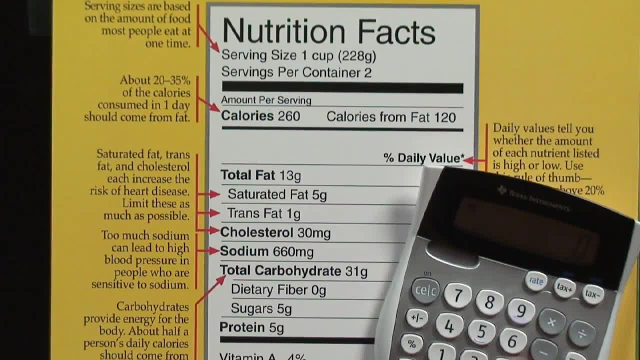 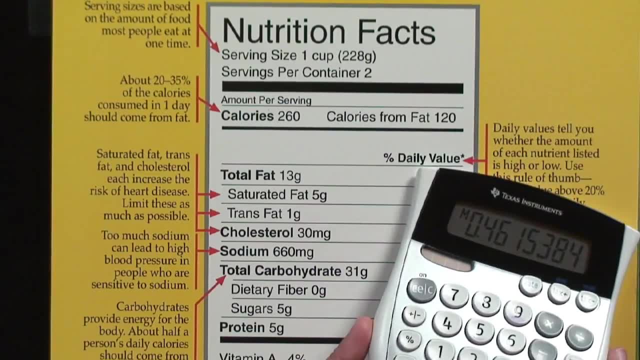 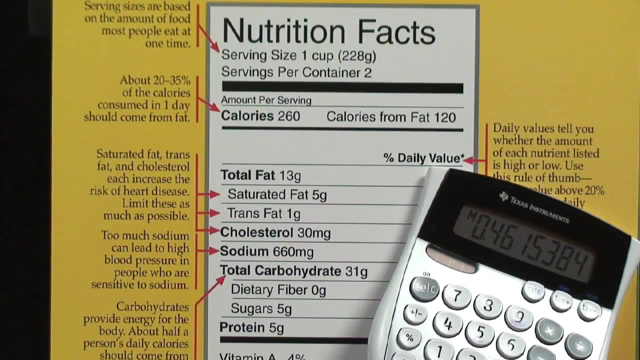 the amount of calories to fat already for us. So we can take a calculator and do a simple percentage calculation. So 120 dividing into 260 equals about 46. This means this product is 46% fat, or 46% of those calories come from fat. Now here we have 5 grams of. 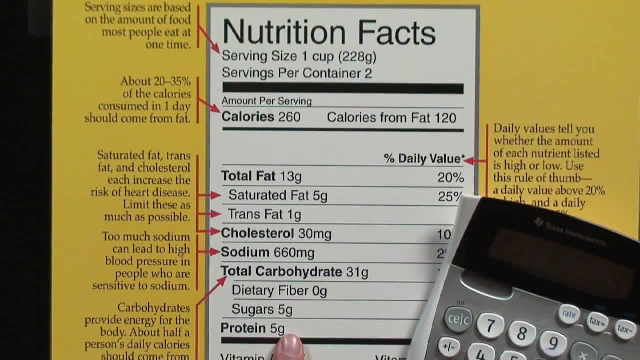 protein. So we know 5,. I'm going to multiply that by 4, because each gram of protein provides us with 4 calories. So I have 20 calories coming from protein. 20 divided into 260 is only about 7 grams of protein. So that's about 4 grams of protein. So that's about. 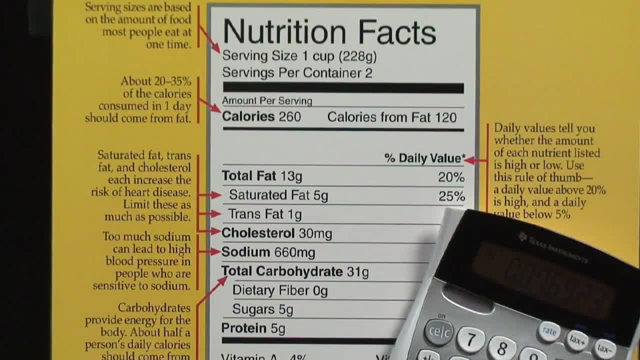 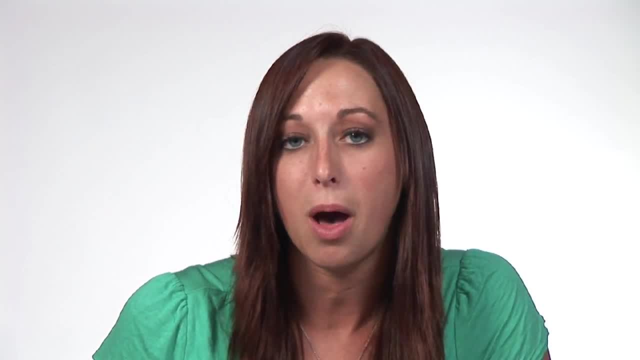 7.6%. So not a significant source of protein here. But again, those are simple ways to find out the percentage of nutrient components per your calories. So how much of those certain nutrient components are providing you calories? But again, as far as daily percent value. 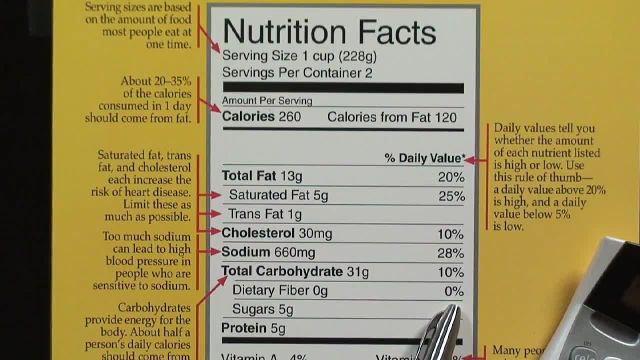 which you can see here. this is based off a 2,000 calorie diet. So if you're aiming for that, 60,, 20,, 30,, like I mentioned, 60% carbohydrates, 20 to 30%, both fat and protein.